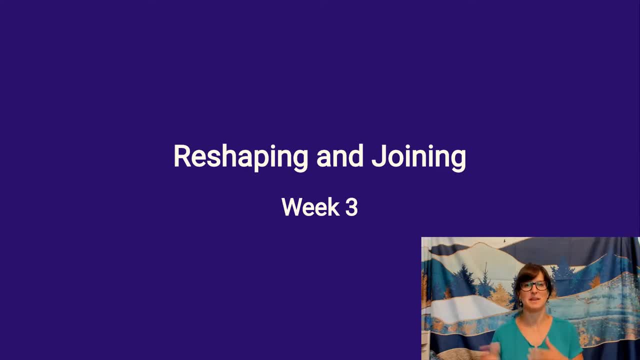 Alright, welcome to week three. So by now you should be a little more comfortable with doing some basic data analyses and using R Markdown to report on these analyses. You should be able to read a data set into R from wherever you've stored it on your computer and you should be able to do some wrangling, some cleaning and some visualizing of that data set. 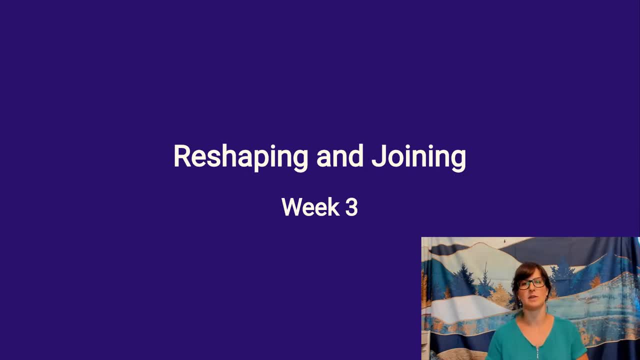 So this week I just want to get a little more complicated with that wrangling process. I want to talk to you about situations where data comes to you in a form that isn't quite what you need for the analysis you want to do, And then we'll talk about some special data types that are a bit more high maintenance and require some special attention. 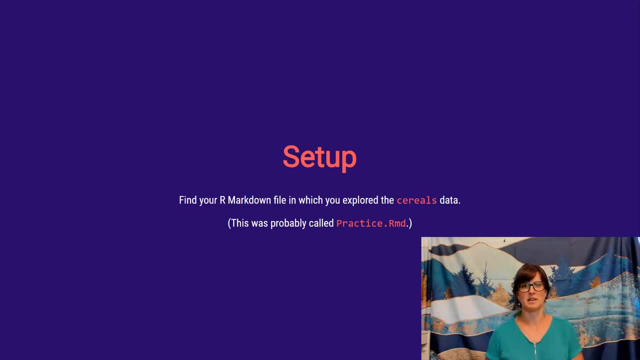 So let's start out with this notion of reshaping. To illustrate this, we'll use that serials data set that you used last week. You probably have this downloaded in a markdown that I gave you called practicermd. If not, you can use this. 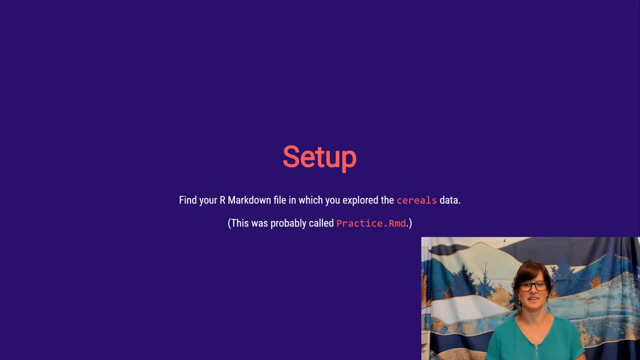 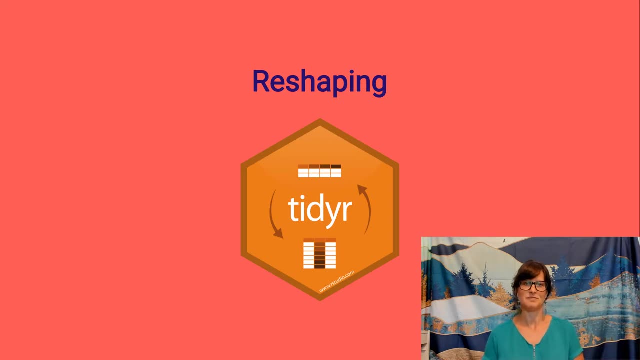 If you can download the data set and read that into your R Markdown file, that's fine too. The package that we're going to use for some of these reshaping tricks is called tidyR. This one loads and installs with the tidyverse, So if you're already installing and loading the tidyverse, you don't have to do anything different. All these functions will already be available to you. 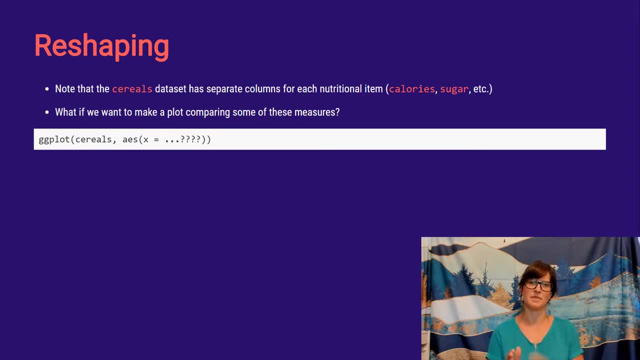 Now notice in this serials data set, the way that it's set up is for each serial. we have many columns measuring each nutritional item, So we're going to do that. So we had a column for the amount of calories in that serial, a column for the amount of sugar and so on. 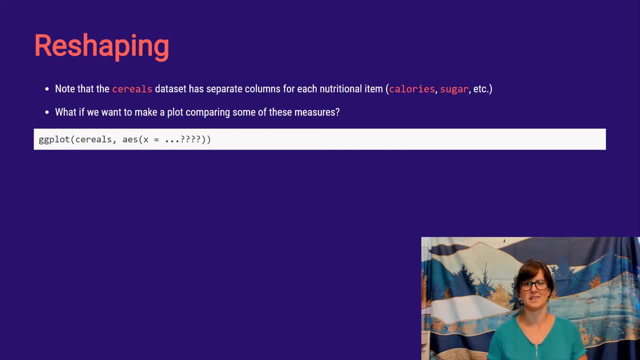 So suppose you said to yourself: well, I would like to make a plot comparing these measures, I would like some box plots showing me how many calories there are versus sugar, versus protein, et cetera, in all of these serials. And so you know already how to use ggplot. and you say to yourself: OK, the first argument is serials. Great, I can do that. 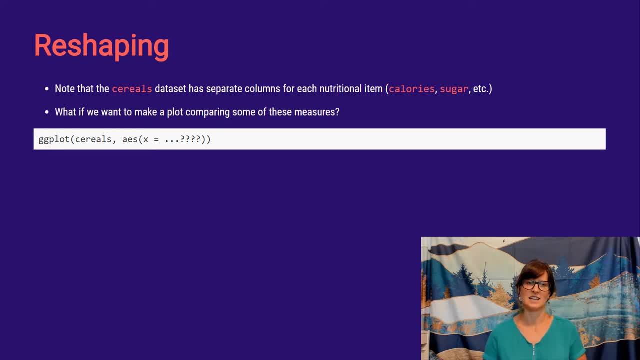 And then you set about defining the aesthetic. And what do you want on the x-axis here? Well, in principle you want that x-axis to be labels for all of those nutritional values. But we can't do x equals calories, because then we just have calories. 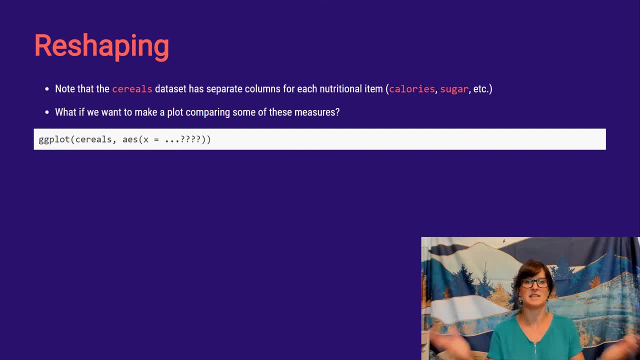 And we can't do x equals sugar, because then we just have sugar And anyways, these are numeric variables, not categorical, So they don't really make sense to be on that x-axis for side-by-side vertical box plots. So we're sort of stuck. 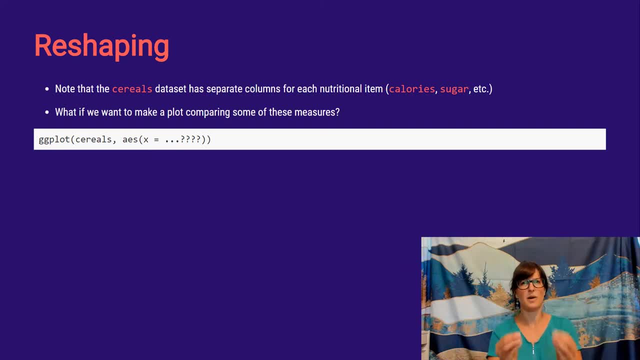 And we're sitting here saying: I know what I want to make, But I don't quite have the data in the form that I want. I don't quite have the data in the form that I need to send that into my grammar of graphics. 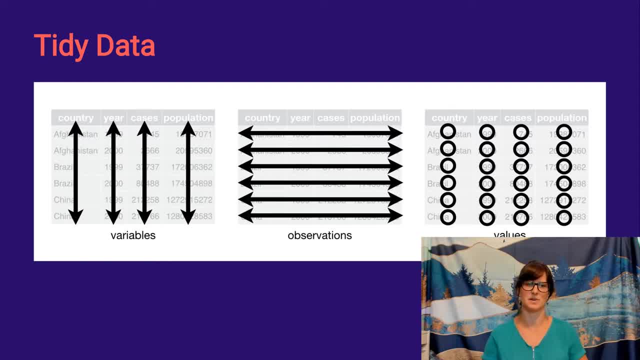 So here is the main concept that maybe will underlie some of this reshaping, And that idea is what's called tidy data. In fact, this is the source of that name: tidiverse for the suite of packages that we've been using. 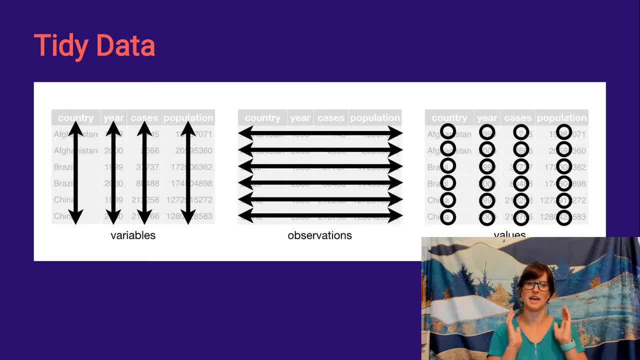 And it's very simple. If data is tidy, then what we have is we have columns that measure variables And then we have rows that represent observations. Maybe these are subjects in a study. like people, These are cereals. These are each of our units of observation. 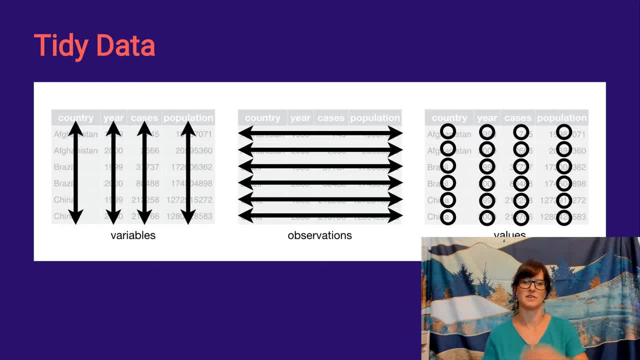 And then the cells within the data set. those are the values. So we have a value for a certain variable observed for a certain observational unit, And this hopefully feels very natural to you, And it's surprising how often you will see data that actually isn't in tidy form and needs to be tidied. 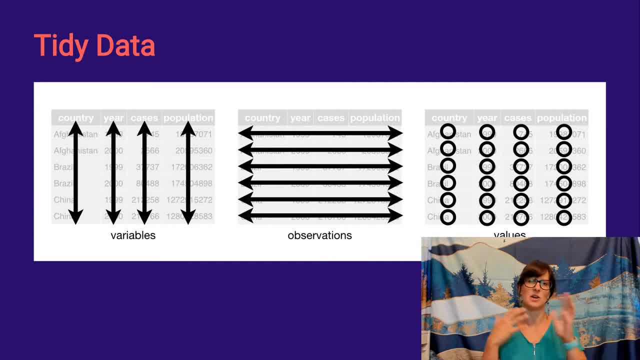 And so I want you to keep this in mind: What are your variables, What are your units And, depending on your analysis, what you think of, as your variables might shift a little bit. So let me show you what happens. So I have this idea that I want to make side-by-side box plots. 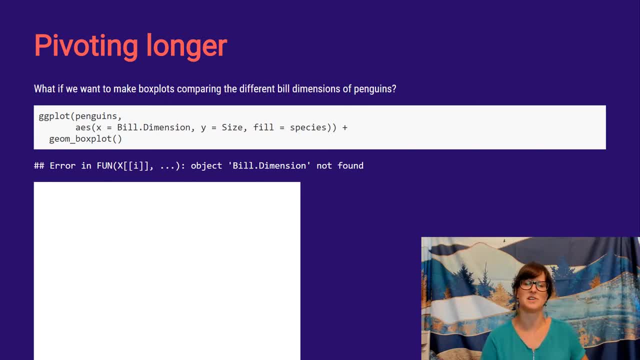 So let's think about that penguin data set again, where we've measured various dimensions of the bills of these penguins, And so I'm trying to make a gg plot with these penguins And I've put the aesthetic that I would like to be able to use. 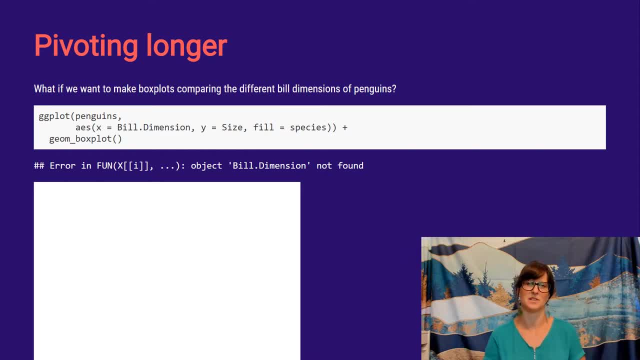 What I think I want to do is I want to have on the x-axis the bill dimension, whether it's the length or the depth of that bill, And then on the y-axis, I want the size And I want the number of millimeters that that bill dimension is measured to be. 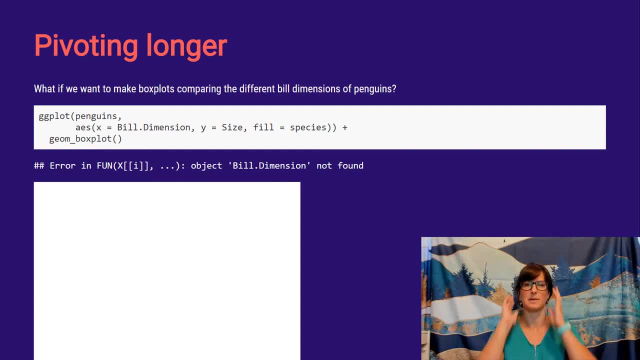 And then I've decided I want to color it by species so I can compare these penguins. And now here's what happens: when I try to make a box plot with that aesthetic, Of course it breaks. We've got a totally blank plot here. 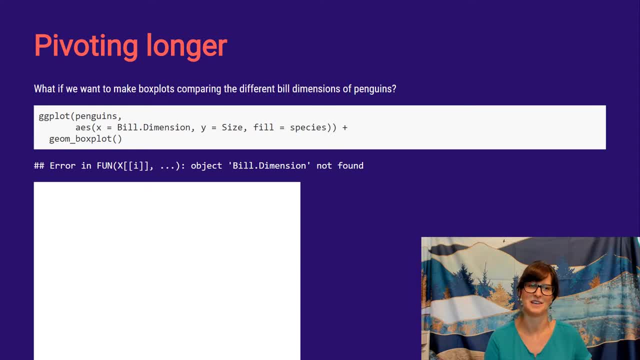 And it says: error: bill dimension not found. Now, if you recall, you can go back and look or you can check out the data yourself- That penguin's data set did not have a variable called bill dimension. What did that data set have instead? 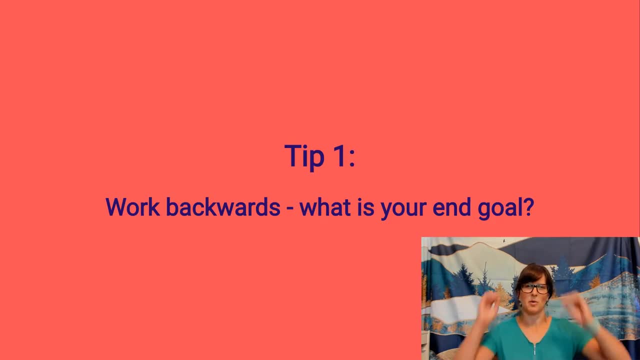 So this is tip number one. I think thinking about these data sets is a little tricky. It requires some shifts in your natural thinking. So here's my first tip of the day. My first tip is to work backwards from your end goal. So if you are trying to make a visualization, or if you are trying to do a certain hypothesis test or a certain summary statistic, 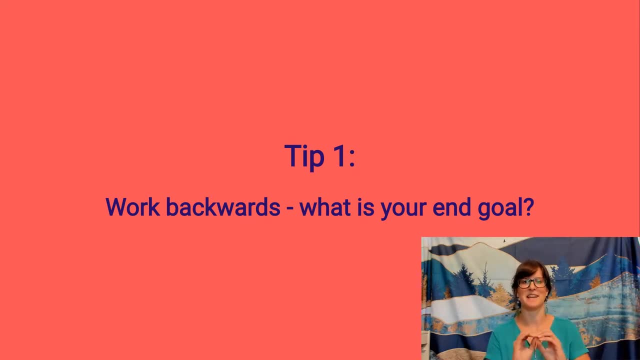 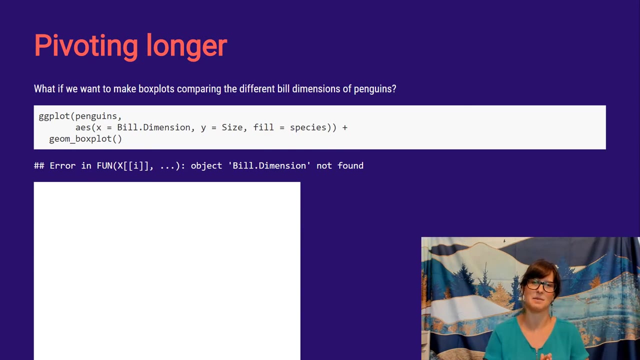 ask yourself: what line of code would you like to be writing at the very end? And so that's what I've done here. I've said. what I really want to do is I want to make the X aesthetic be bill dimension and the Y aesthetic be the size. 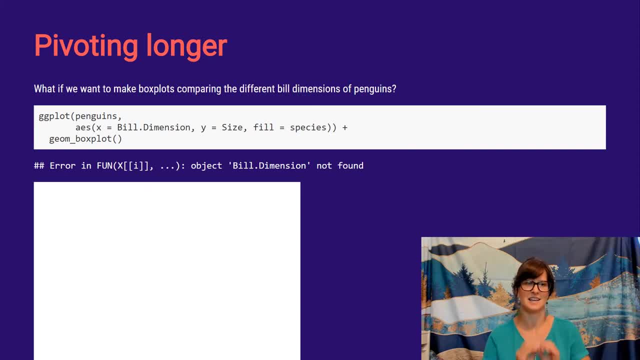 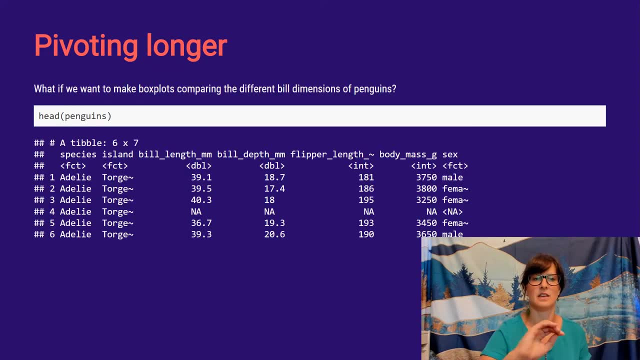 Even though those variables don't right now exist in my data set. that's what I would like to have in the end of my process. So now I've defined my end goal. So let's take a look at this data frame. So here we have our penguin's data frame. 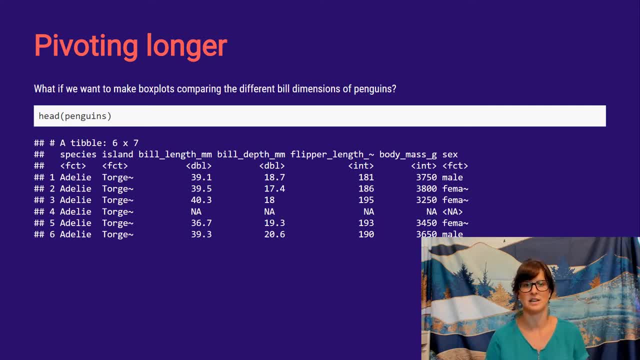 And we can see that none of these variables is called bill dimension. We do have bill length and bill depth And we have numbers for each of these. So I have to ask myself: how can I morph this data set, How can I reshape this data set in order to have the same information but formatted with bill dimension and size as two different variables that I can put into an aesthetic? 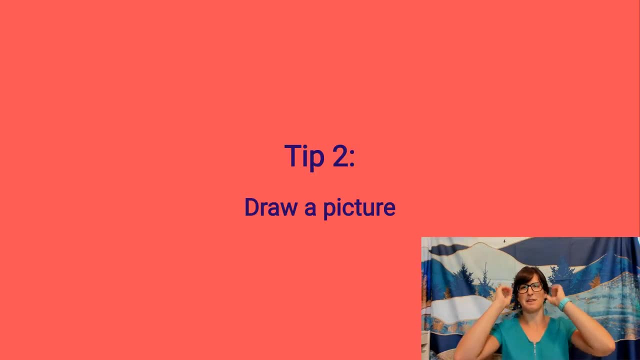 So my second tip of the day- and this is my favorite thing to say in almost any class- is: draw a picture. I literally mean not just draw a picture of the plot you're trying to make. Draw a picture of the data set that you are trying to create. 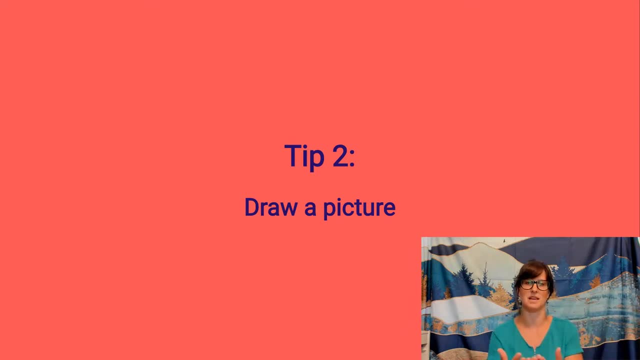 Draw a picture of what form you would like that data to be in, so that you can get to your end goal. final step: So, now that we know what we're aiming for, now that we have an idea of what our variables are in that tidy data set and what information they contain, 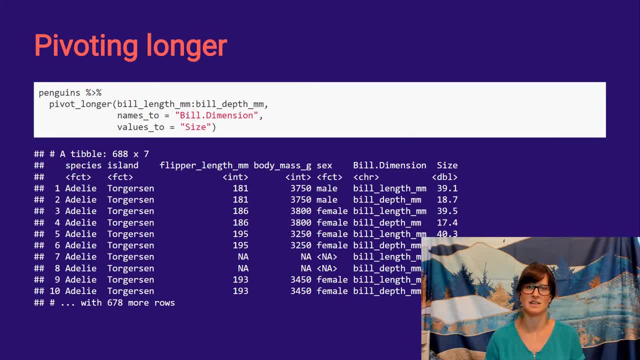 now I can think about using code to achieve that. So in this case, the function I want to use is called pivotLonger, So I'm taking my data frame, which currently is wide. It has the dimensions of the bill as different variables. 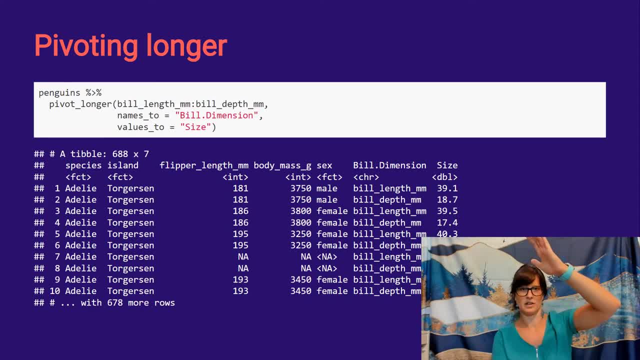 And I'm going to pivot that thing to be long so that now I have each dimension listed with its corresponding size. So the original variables that I wanted to take from wide to long we can see right here. Those were billLength and billDepth. 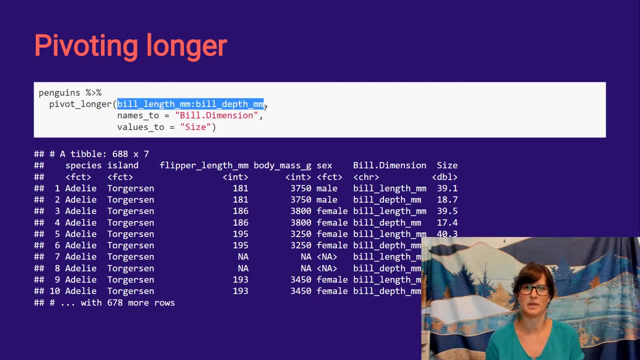 Now you could pivot more than two variables. In this example it's just two. And then we say, alright, what am I going to do with that information? Well, I want to take those original variable names and store them in a new long column called billDimension. 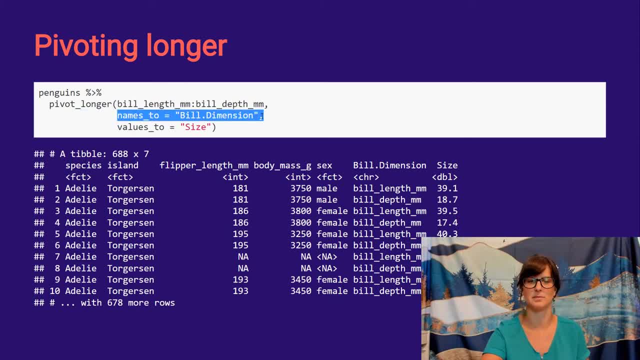 So that's that first argument here names to billDimension And we can see in the final product that's what happened. Here's a column called billDimension And it has billLength, billDepth, billLength, billDepth. This is a categorical variable saying which dimension I am currently measuring. 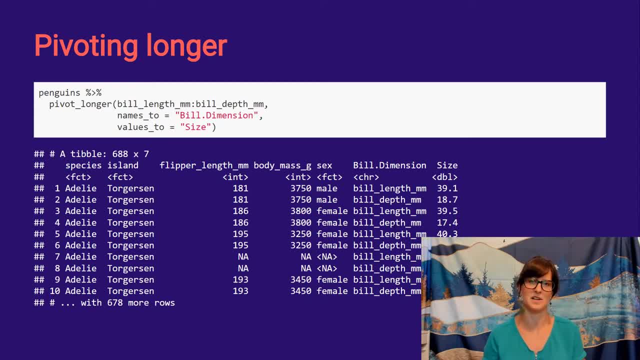 And then I said, well, what do I want to do with those original measurements of length and depth? Where do I want to put those values? I want to put those values. I want to put those values in a column called size. So here I have, for the first penguin. we have some demographic information. 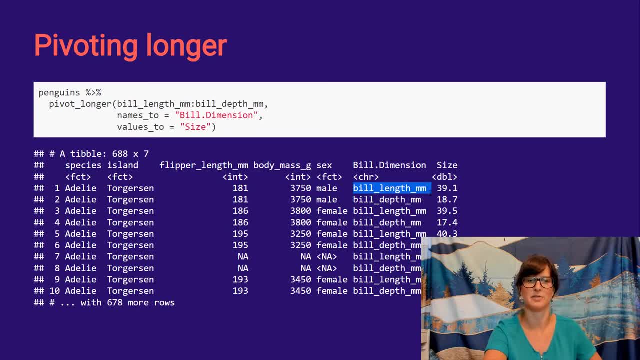 And then we see that the billLength of that particular male Adderley penguin from Torgerson was 39.1 millimeters, And for the exact same penguin- so he's listed twice- that billDepth is 18.7.. 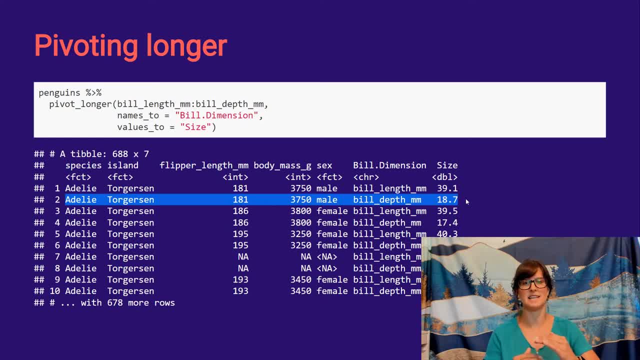 So now, instead of each penguin being listed once, we've got them listed twice. It's kind of a long data set. Our idea of observations has changed a little bit. Now it's not that each row is a penguin, It's that each row is a bill dimension of a penguin. 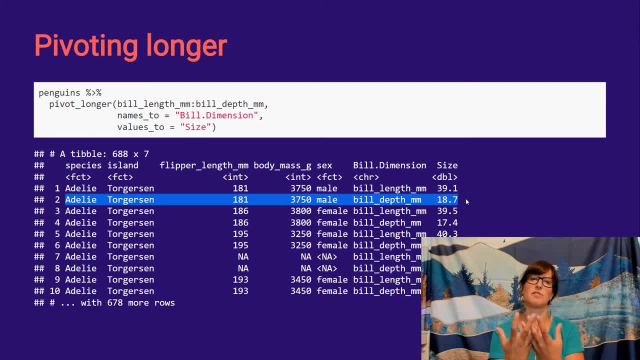 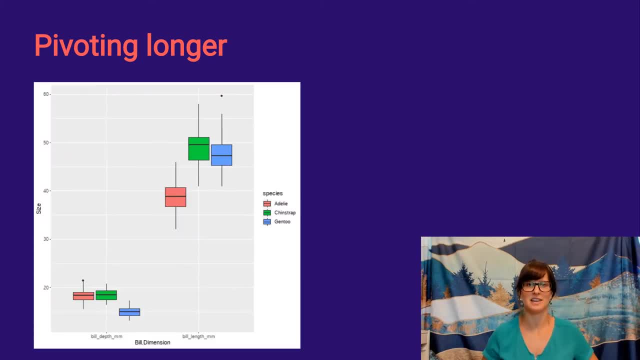 But other than that, it's the exact same information. It has just been morphed into a different shape for the data set. And so, now that we have the data set looking how we want it, that original code, that aspirational ggplot code. 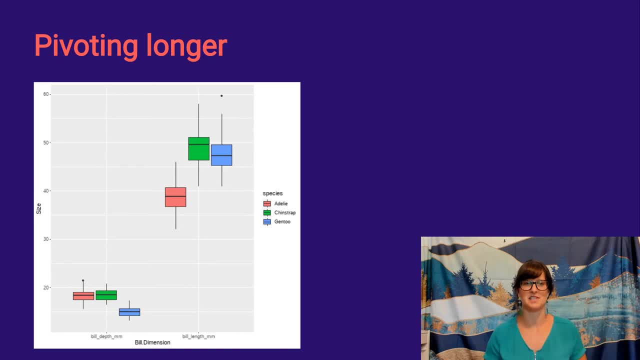 will produce a picture like this: We've got our bill dimension on the x-axis, our size on the y-axis. So now these two bill dimensions- depth and length- have been separated, And then we have boxplots colored by each of the three species. 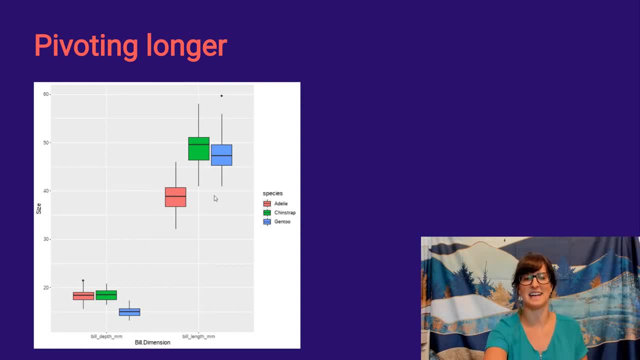 And this gives us some takeaway message. We can see here that this Adderley species maybe has a slightly shorter bill, but not necessarily a shallower bill. The shallower bill is the Gen 2 penguin, And so if you know a little bit about penguins, I suppose 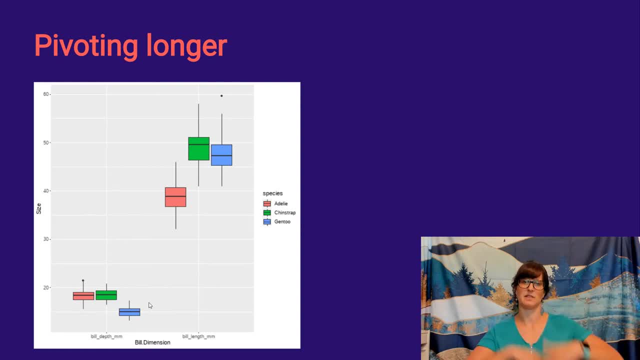 this might give you a better idea of what's going on with these species. We have reshaped our data so that we can make the visualization that was our end goal for the analysis. Now I want to let you know about something really quickly. This pivotLonger function is a little new. 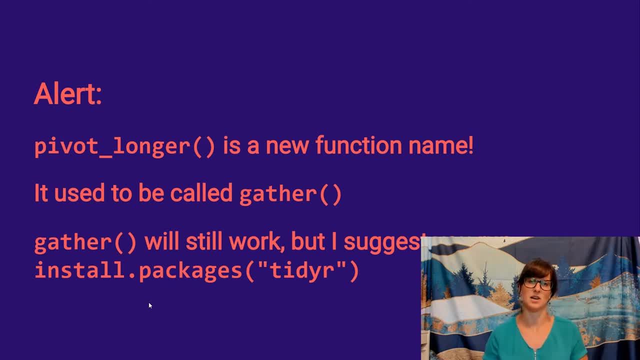 It came about maybe six months ago. This function used to be called gather. So if you see old code that uses the word gather, or maybe if you have an older version of TidyR installed, you may be more familiar with gather, And that's okay. 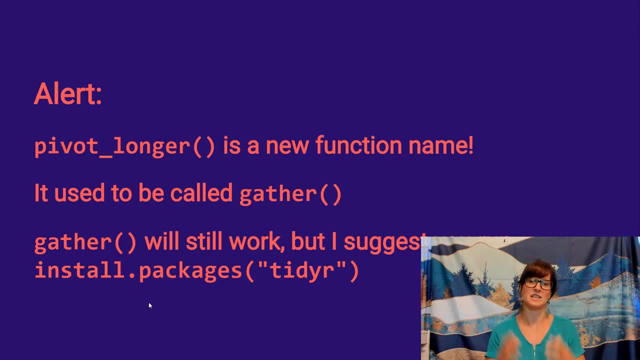 I think the pivotLonger function is a bit clearer and easier to use. personally, I do suggest that you reinstall TidyR in order to update that package and get this new version pivotLonger. But don't get too confused If you see gather same idea. 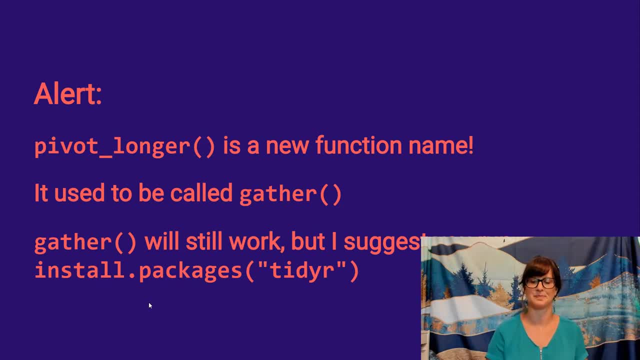 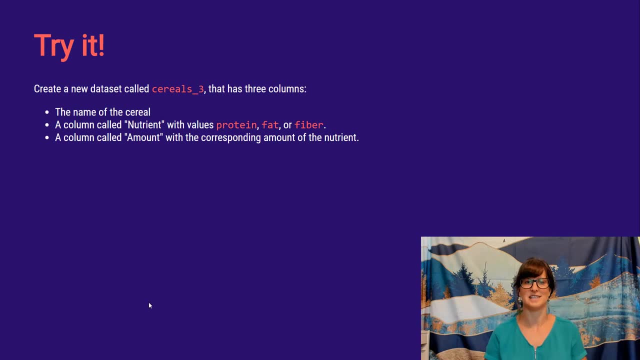 It is reshaping the data to be longer instead of wider, So this is your chance to try this out on your serials data set. So I want you to create a new data set. Let's call it serials3, since we did 1 and 2 last week. 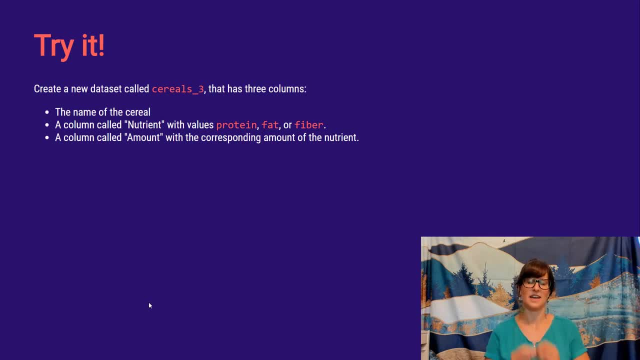 And what I want is the name of the serial. And then I want a column called nutrient And I want a column called amount, And you can narrow this down to just protein, fat and fiber. I don't need all of the nutrients. 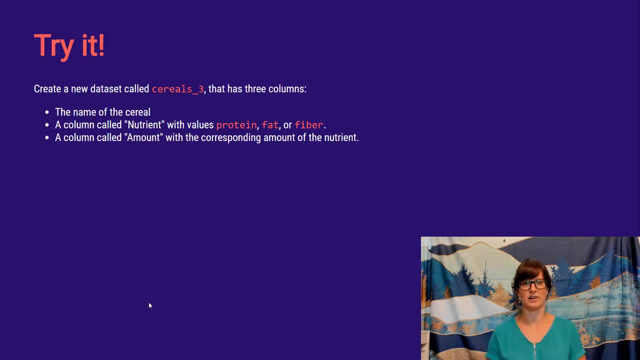 It just needs to be pivoted. So see if you can apply what you just learned in order to take that wide serial data with so many nutrients listed as columns and make it a long data set with these two variables: nutrient and amount. I'll give you a moment to do that. 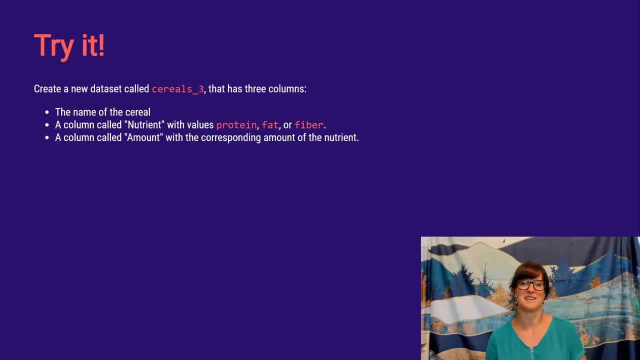 Okay, So hopefully you took a minute and tried that out and hopefully successfully pivoted your data. If you're one of those people who's not pausing the video and trying these things, really you're just hurting yourself, So I really recommend that you take a moment pause. 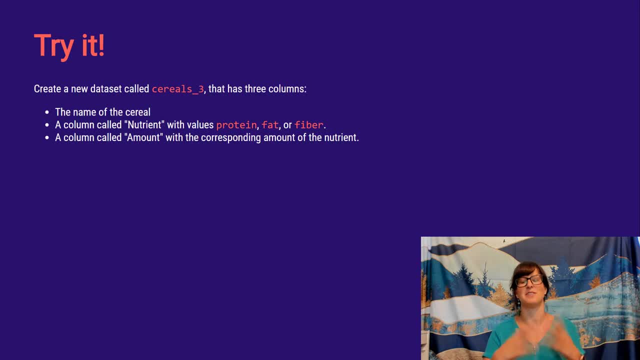 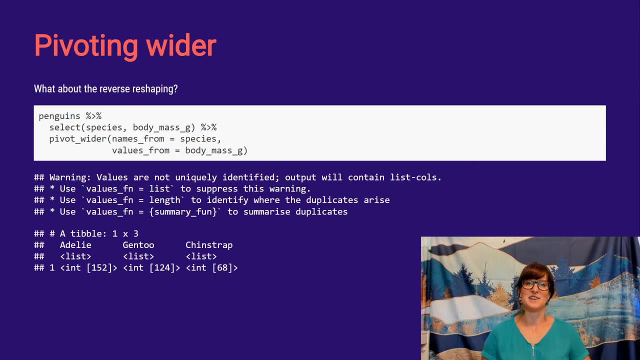 and actually try this out. It's not enough to look at code. You need to learn by doing. You need to type your own code. But regardless, let's move along. Now. you might say to yourself: okay, if I can take a data set that's wide and make it long. 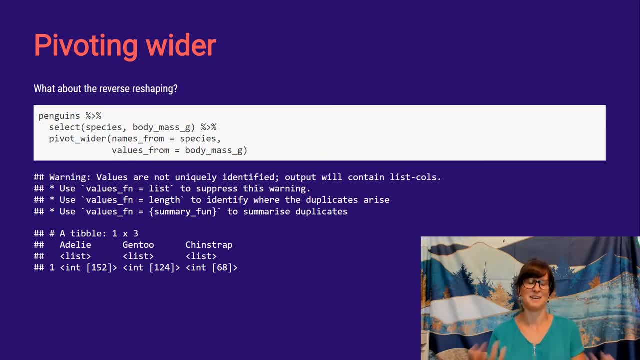 surely I can take a data set that's long and make it wide, And of course you'd be right. That function, as you might guess, is called pivot wider. And now, instead of taking variable names and sending them to a column, 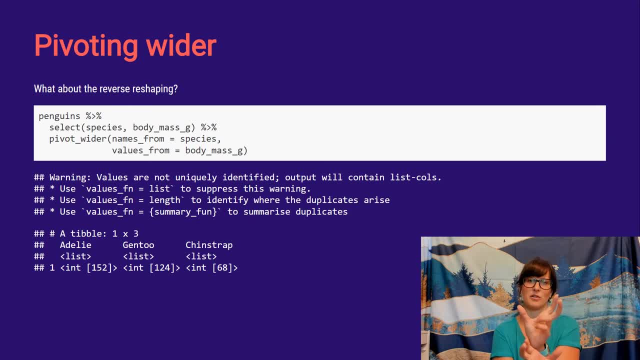 we're taking an existing column- hopefully one that has a categorical variable, that has words, and sending those to be new column names. So here we have our three species, Adelie, Gentoo and Chinstrap, And what we'd like to do is take this data frame. 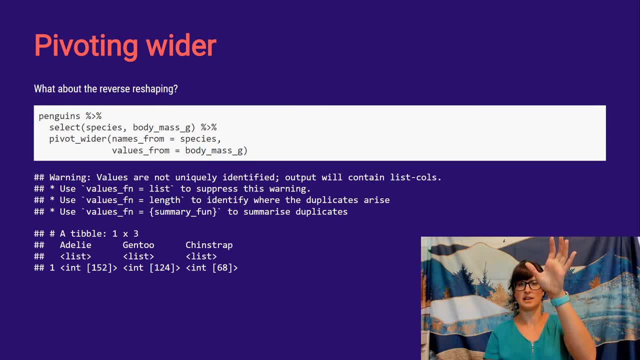 that has one column called species, with those three categories, and turn it into three separate columns. And then, what do we want to put in each of those columns? Well, in this case I've chosen the variable body mass, So what I'd like each of those columns to have. 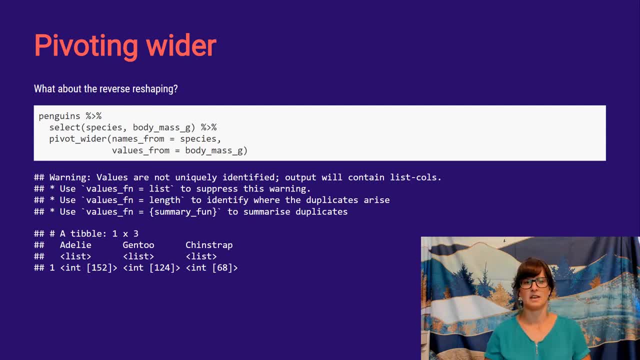 is the body mass of that penguin. Now this looks like this code should work, but instead we get this strange warning here, And R tries to do its best. Remember that a warning is not an error. It says I tried to run this code. 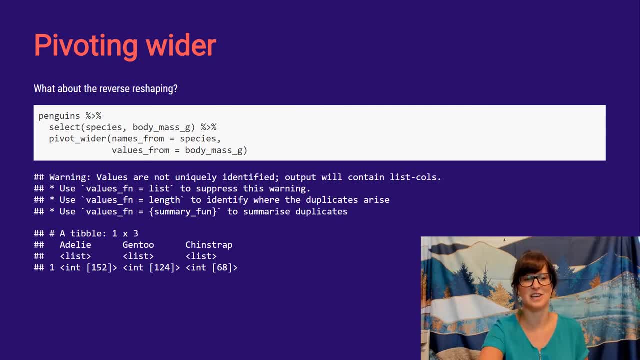 But what it gives you here is this strange-looking data frame where the Adelie column contains, within the column, a list. So each element of that variable is itself a list, And so we've got one list for Adelie, one for Gentoo. 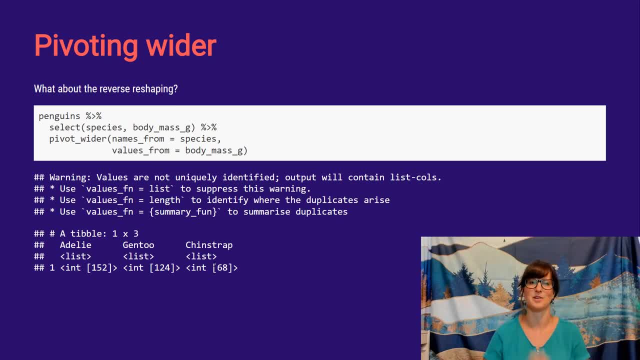 one for Chinstrap. It's strange. It's unhelpful. You probably don't know how to work with this data. What's going on here is that when we pivot wider, we need a column that identifies the individual penguins. There's a nice shortcut function for this in the tidyverse. 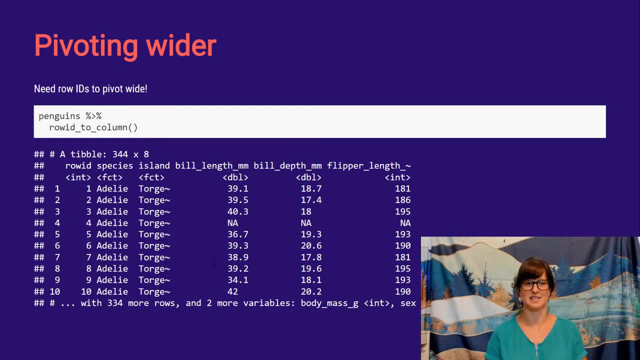 row ID to column. There are many other ways to create this column if it doesn't exist, And so here, what I've added on is not just the demographic information of each penguin, but I've given each penguin a label, just a number. 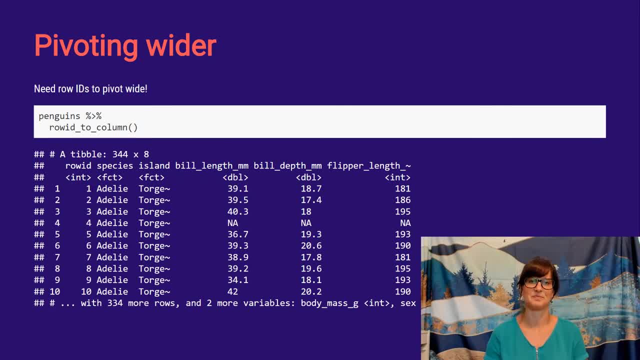 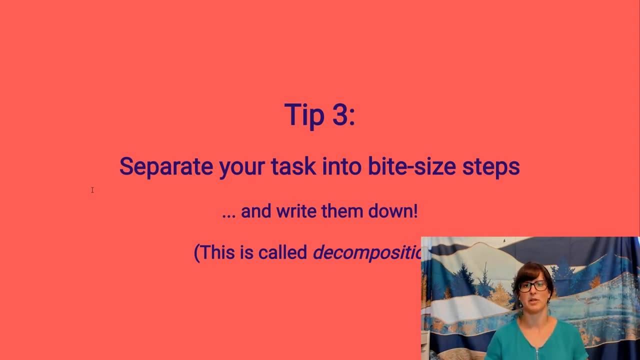 one through 344.. And why this is necessary is because then, when we pivot wider, we can keep track of which values in the new columns corresponded to which penguin. So this leads me to my tip number three for thinking about reshaping. 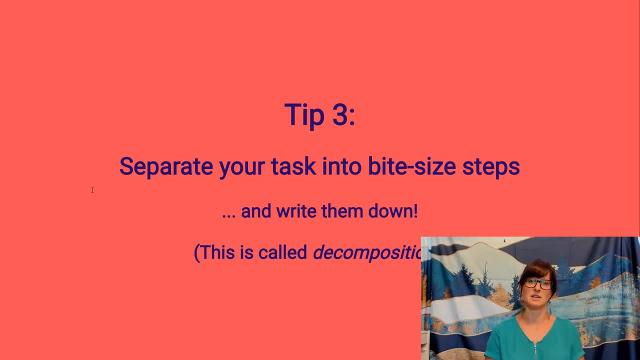 which is to separate your task into bite-sized steps. It can be very easy to think of your end goal, work hard, figure out that end goal and then try to do everything all in one blow. This is difficult for troubleshooting and this is difficult for making nice pipelines. 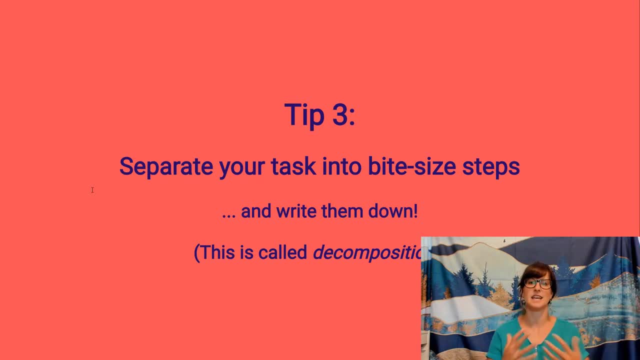 So I want to encourage you to do what's called decomposition, to take your task and write it out as bite-sized steps. In this case, my steps were: create an identifying column, then pivot the data and then maybe I visualize or analyze the data. 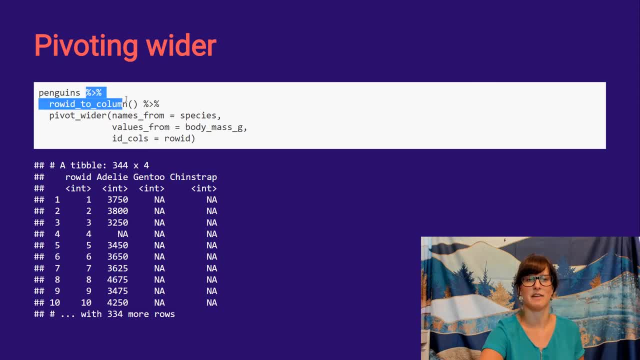 And so in this case, this is what the pipes are great for. I'll go through that first process of adding the row ID to column. I don't have to save that new variable into the data set. Notice, here I didn't update the penguins data set at all. 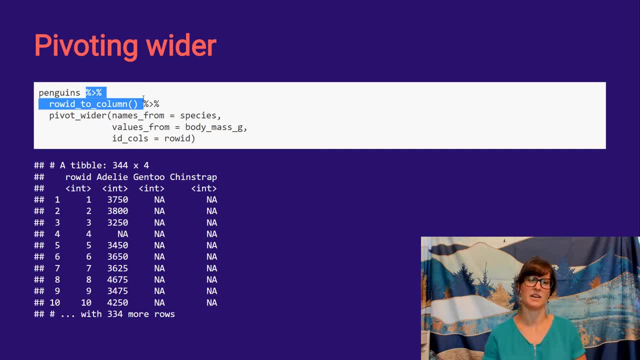 because I don't really need that new variable to always be there, I'm just using it for this pivoting process. And then I take that result and now I pipe it into pivot wider. And there we go, We have pivoted wider. 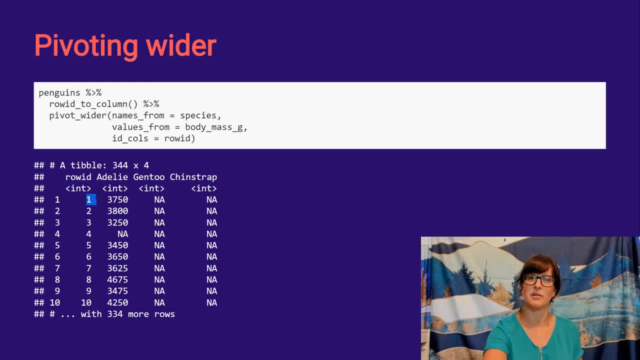 And so we've said: here's penguin number one. Penguin number one is Adelie, So we have its body mass in the Adelie column And penguin number one is Adelie. And penguin number two is not a Gen 2 or chinstrap penguin. 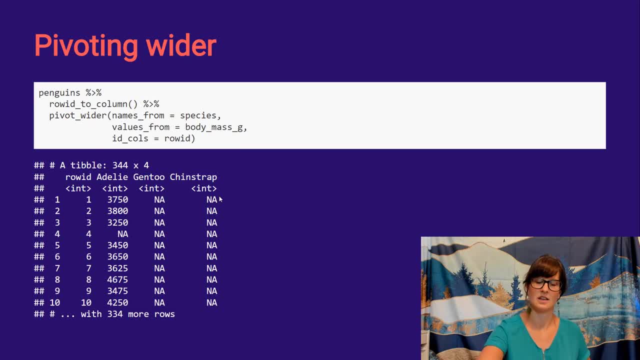 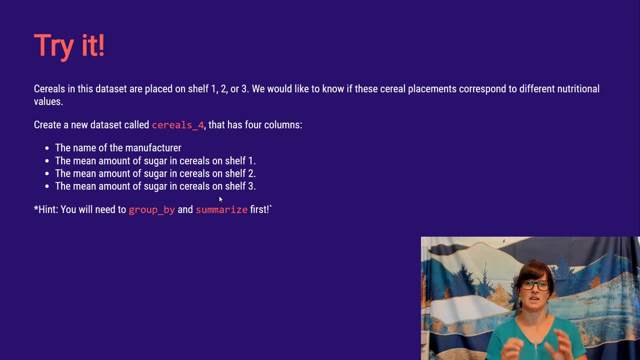 And so this just fills in with NAs. So let's try this out on some data where pivoting wider makes a little more sense than the penguins data. In your cereals data set you have a variable that tells you which shelf that cereal was placed on: one, two or three. 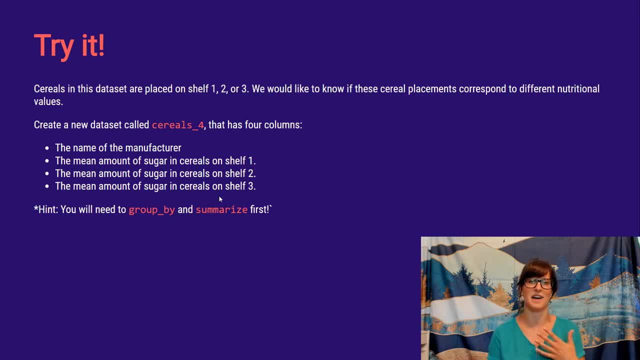 And I'm interested to know: do these cereal placements correspond to different nutritional values? For example, maybe a very sugary cereal for those children might be placed on a lower shelf, so the kids will see it. So I want you to make a new data set. 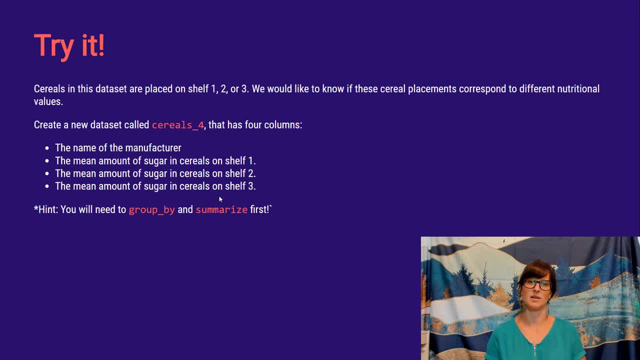 We'll call it very creatively: cereals four, And I want four columns. I want you to give me the name of the manufacturer. I want you to give me the average amount of sugar for cereals from that manufacturer on shelf one. That was a lot of qualifiers. 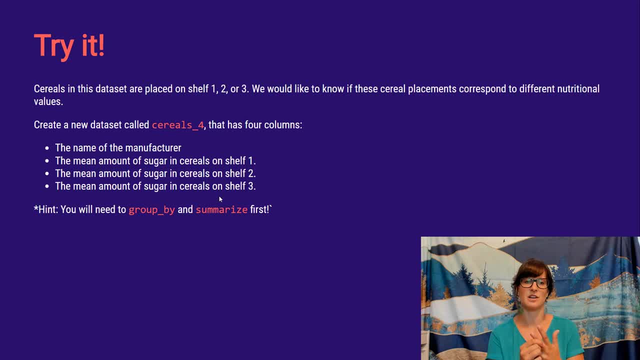 The second column is the mean amount of sugar among all cereals in that manufacturer who were put on shelf one, And I want you to give me the average amount of sugar from that manufacturer on shelf two. This is going to take you several steps.